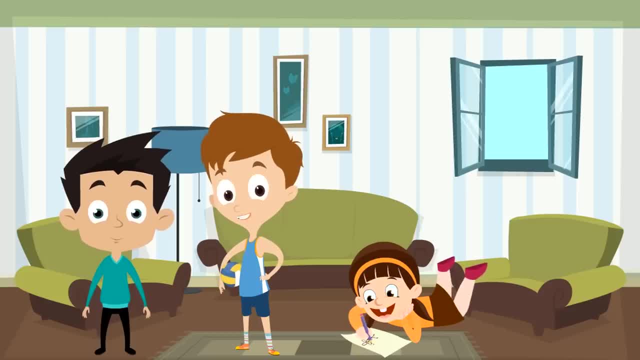 Now in Ethan's house there are only three carrots. They're just three carrots. We are going to have to divide the three carrots amongst the three kids. So let's figure this out. How many carrots does each kid get? Do you know? 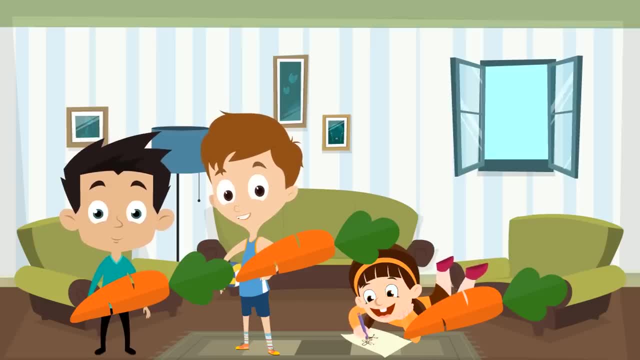 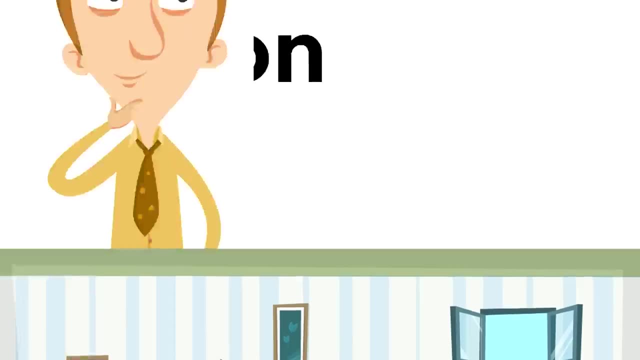 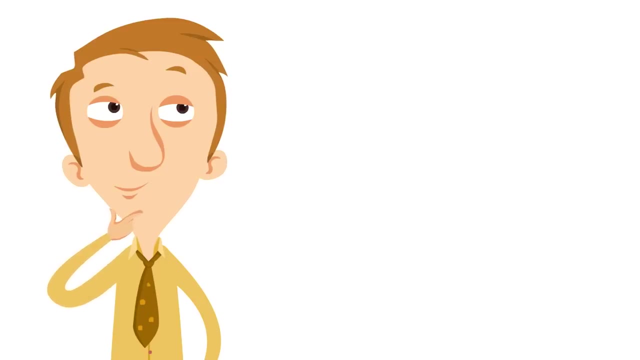 Uh-huh, Each kid gets one carrot. Pretty simple, right? Three carrots, three kids. Each kid gets one carrot. Hey did you know? we just did division. Uh-huh, We just did division. Division is pretty simple. You see, division is splitting a number up by any given number. 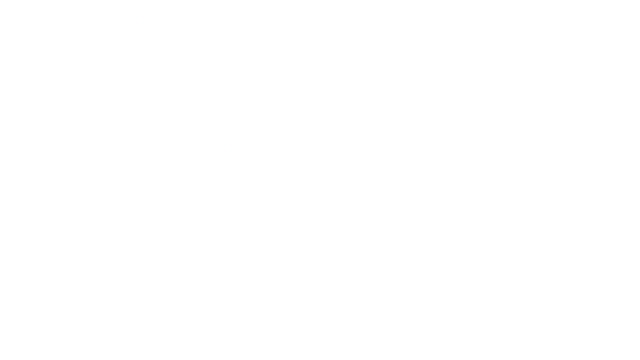 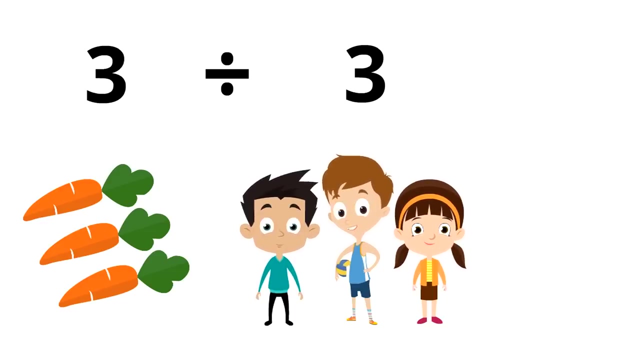 That's it Just splitting a number up. Let's look at our story again. There were three carrots and we divided those three carrots by three because there are three people, right, The three kids that love carrots, And the answer of how many carrots each kid gets is one. 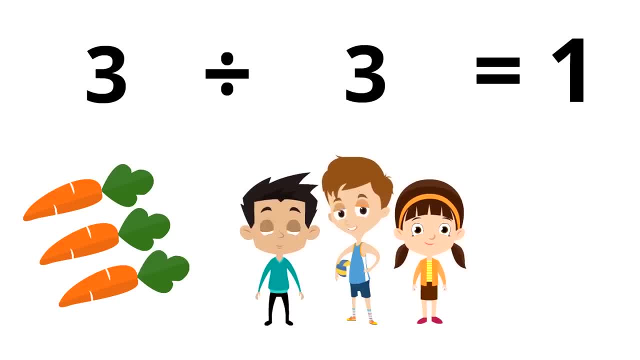 Three divided by three equals one. Notice, right here is the division sign. This is what it looks like When you see that sign. you could just say: divided by. So this reads: three divided by three equals one. Divided by three equals one. 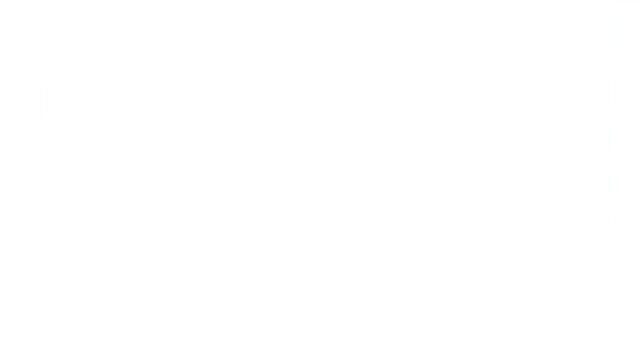 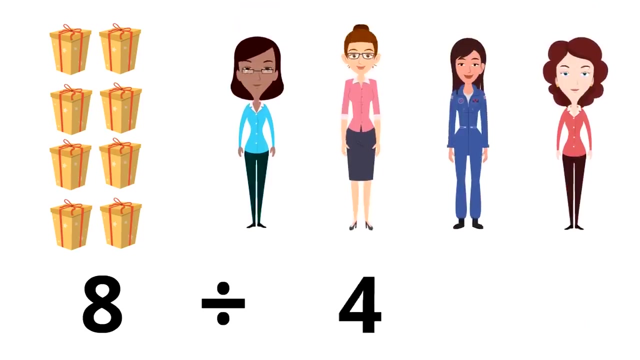 Let's try another example of division. Let's say there are eight presents, Eight presents, and there are four women and we want each of the women to get the same amount of presents as the other women, because we want it to be fair. Notice the division sign. We are going to divide or split up eight by four. 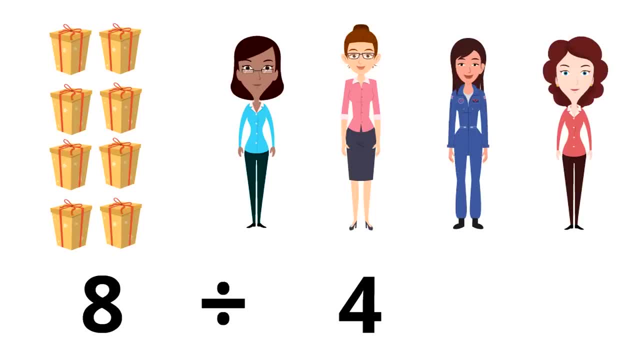 Remember: to divide is to split up. Let's split these presents up into four equal groups: One, two, three, four. Alright, how many presents does each woman get? Uh-huh two. Each woman gets two presents. Isn't that cool. Division is so much fun and it's so easy. 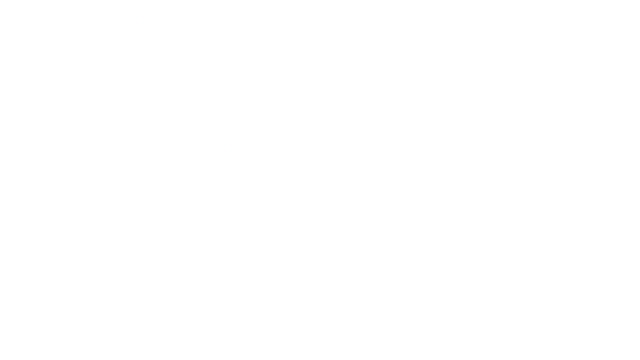 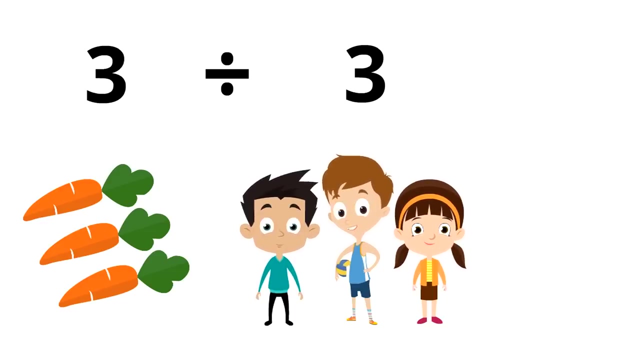 That's it Just splitting a number up. Let's look at our story again. There were three carrots and we divided those three carrots by three because there are three people, right, The three kids that love carrots, And the answer of how many carrots each kid gets is one. 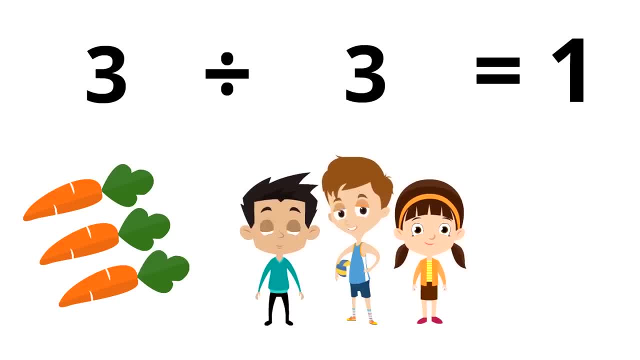 Three divided by three equals one. Notice, right here is the division sign. This is what it looks like When you see that sign. you could just say: divided by. So this reads: three divided by three equals one. Divided by three equals one. 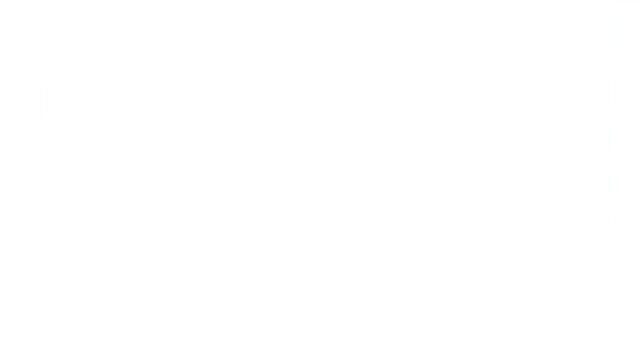 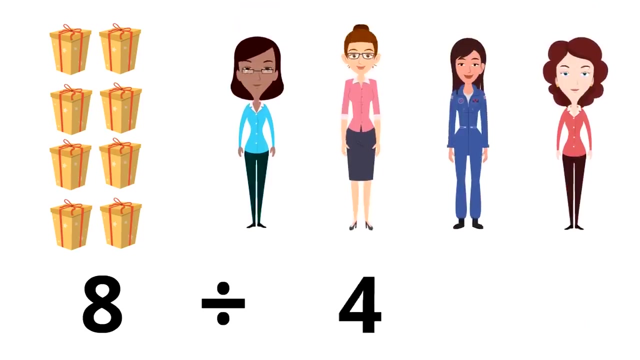 Let's try another example of division. Let's say there are eight presents, Eight presents, and there are four women and we want each of the women to get the same amount of presents as the other women, because we want it to be fair. Notice the division sign. We are going to divide or split up eight by four. 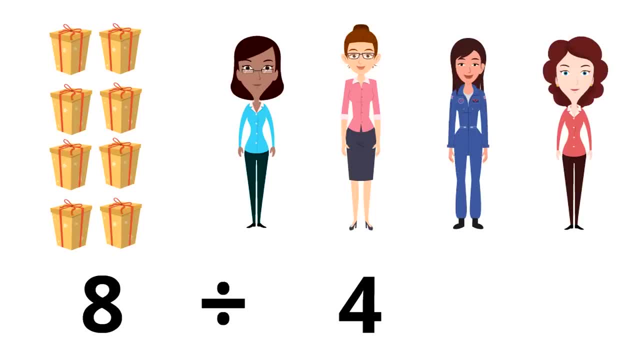 Remember: to divide is to split up. Let's split these presents up into four equal groups: One, two, three, four. Alright, how many presents does each woman get? Uh-huh two. Each woman gets two presents. Isn't that cool. Division is so much fun and it's so easy. 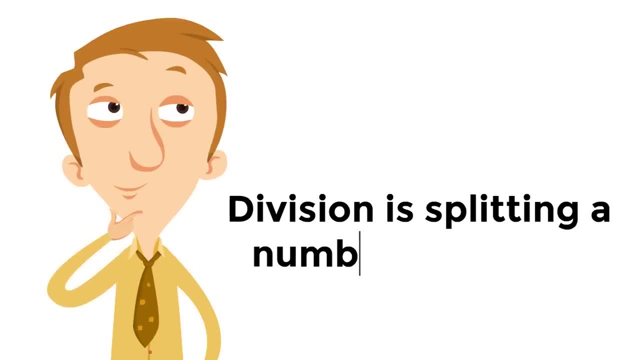 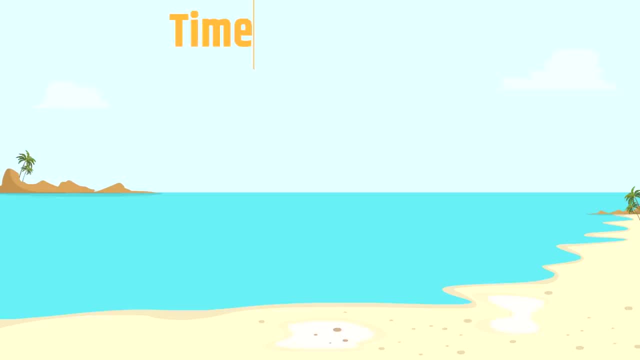 Remember, Division is splitting a number up by any given number. That's it. Alright, now it's time for division facts. We're going to learn some pretty interesting facts about division, And you're going to be like what? Oh my goodness. 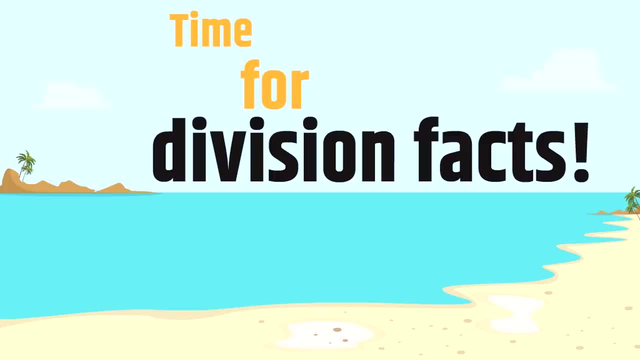 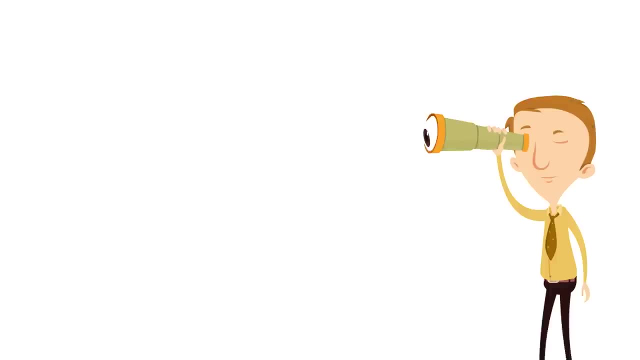 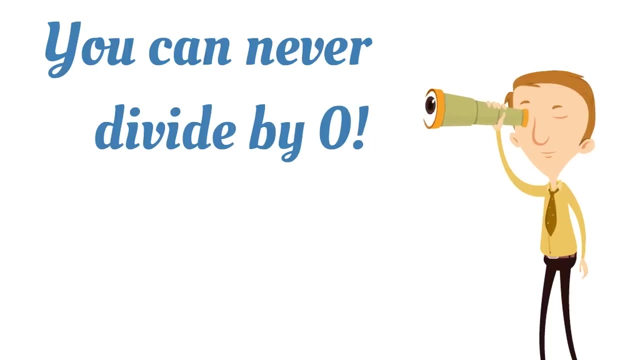 Like secrets. This is super cool, okay, So just look around. alright, Make sure, Are those clear? Alright, It's time for division facts. The first fact is this: You can never divide by zero. It's true, You can never divide by zero, even if you're a rule breaker and you're like 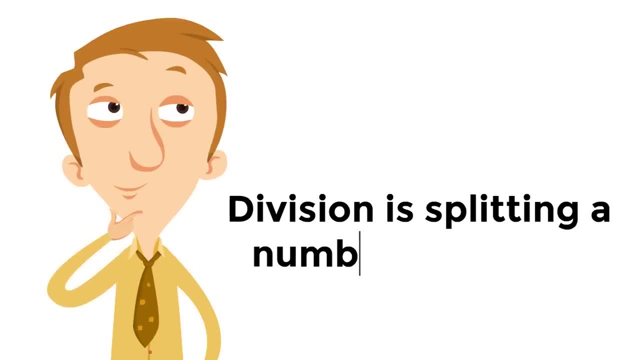 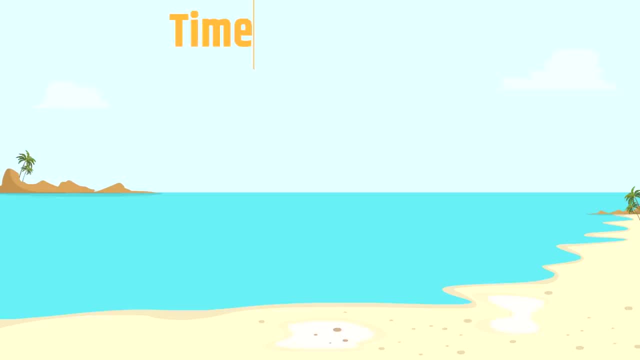 Remember, Division is splitting a number up by any given number. That's it. Alright, now it's time for division facts. We're going to learn some pretty interesting facts about division, And you're going to be like what? Oh my goodness. 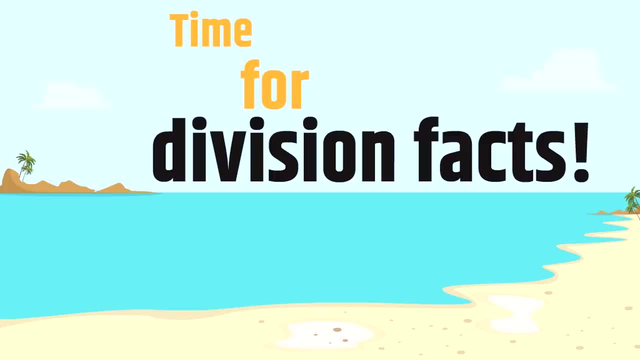 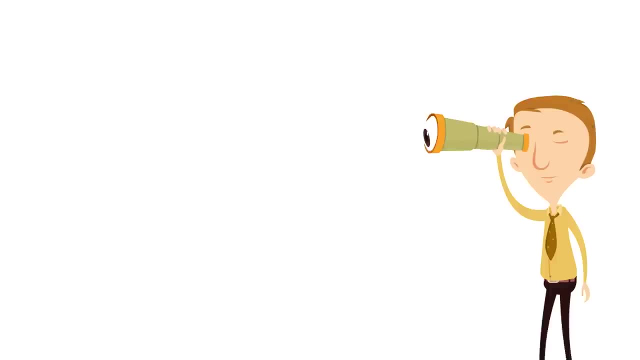 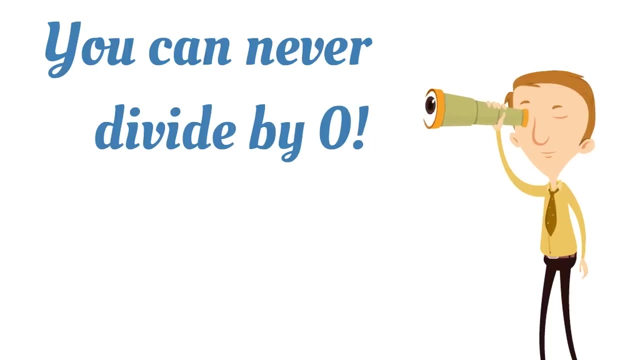 Like secrets. This is super cool, okay, So just look around. alright, Make sure, Are those clear? Alright, It's time for division facts. The first fact is this: You can never divide by zero. It's true, You can never divide by zero, even if you're a rule breaker and you're like 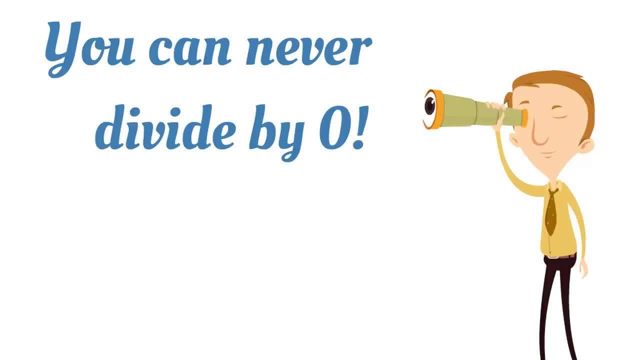 I'm going to do whatever I want. You still can never divide by zero. In fact, if a teacher ever gives you a test and you see a problem where you have to divide a number by zero, just write on the test: undefined. 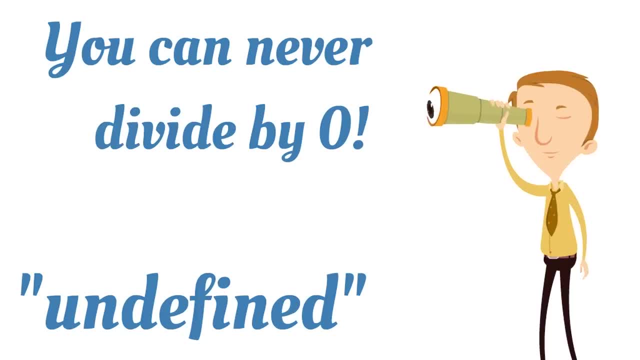 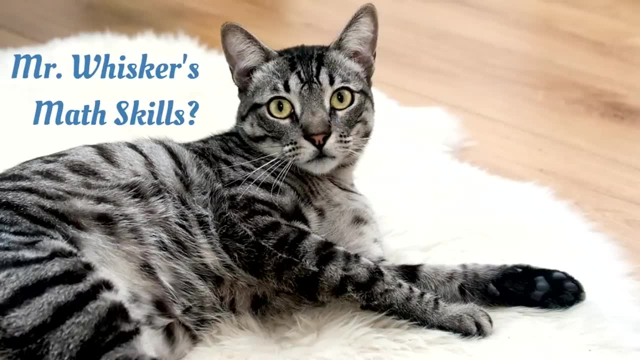 Because that's exactly what that answer would be Undefined, It's impossible. Kind of like Mr Whiskers' math skills. Does Mr Whiskers do math in his head all day long? Who knows? His math skills are undefined. 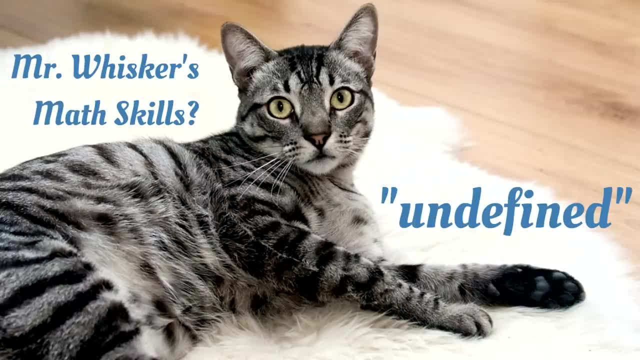 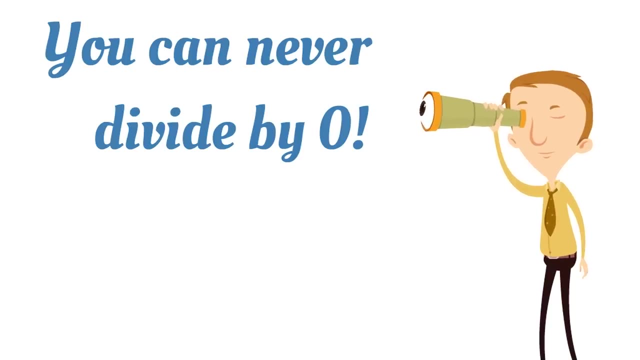 We just don't know. It's impossible to know. You know Mr Whiskers might know how to do division, Who knows? Undefined. You can't divide by zero. You can never divide by zero. If you ever see any division problem dividing by zero. 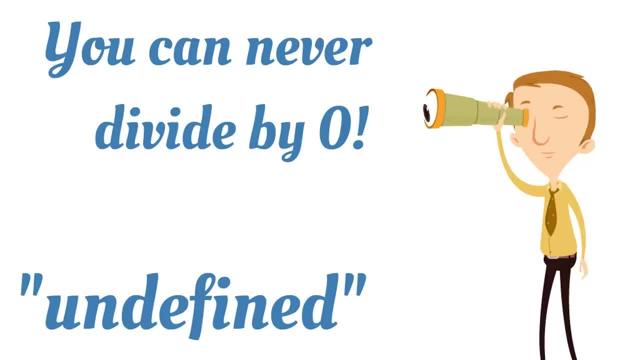 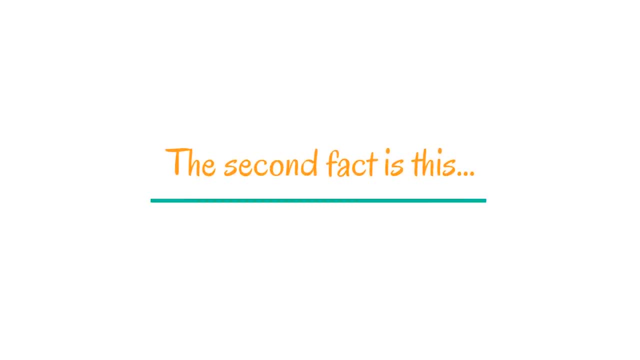 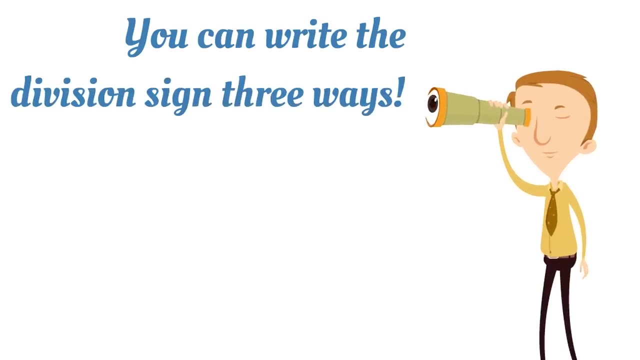 just write undefined. It's impossible. It's impossible, So just write undefined. The second fact is this: You can write the division sign three ways. Uh-huh, Not just with that traditional division sign. You can write it like the division sign. 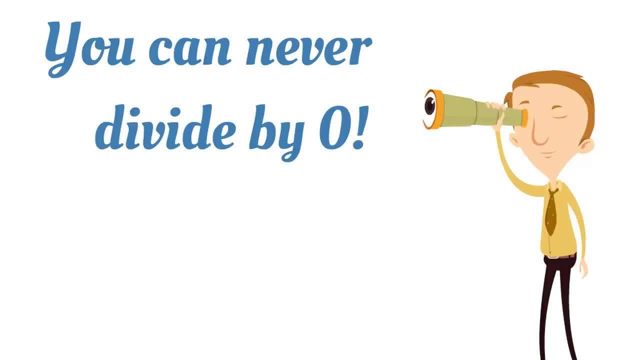 I'm going to do whatever I want. You still can never divide by zero. In fact, if a teacher ever gives you a test and you see a problem where you have to divide a number by zero, just write on the test: undefined. 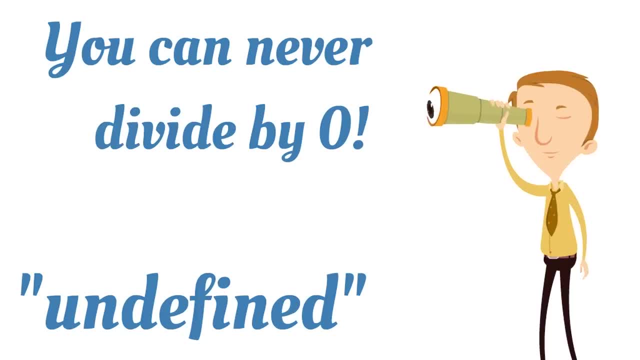 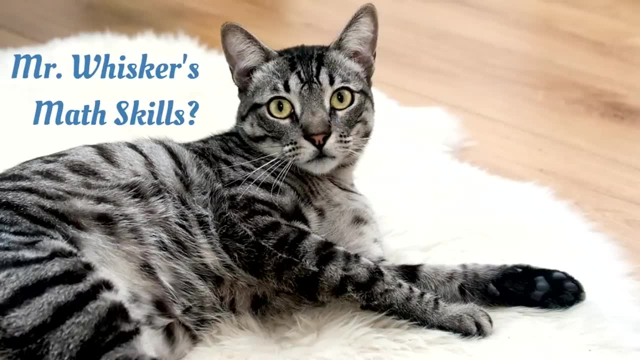 Because that's exactly what that answer would be Undefined, It's impossible. Kind of like Mr Whiskers' math skills. Does Mr Whiskers do math in his head all day long? Who knows? His math skills are undefined. 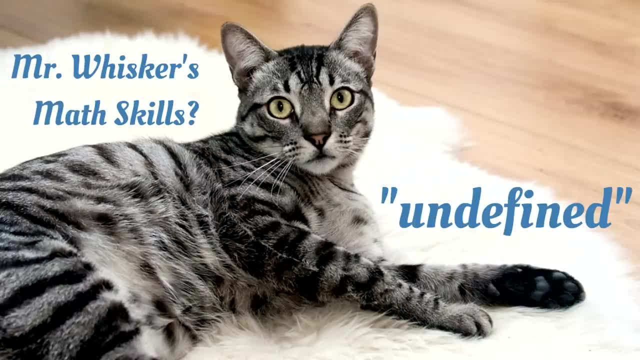 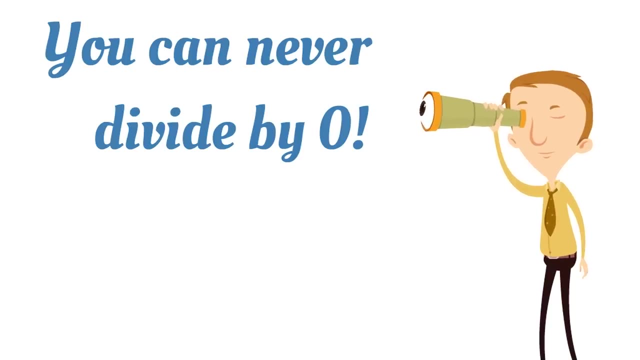 We just don't know. It's impossible to know. You know Mr Whiskers might know how to do division, Who knows? Undefined. You can't divide by zero. You can never divide by zero. If you ever see any division problem dividing by zero. 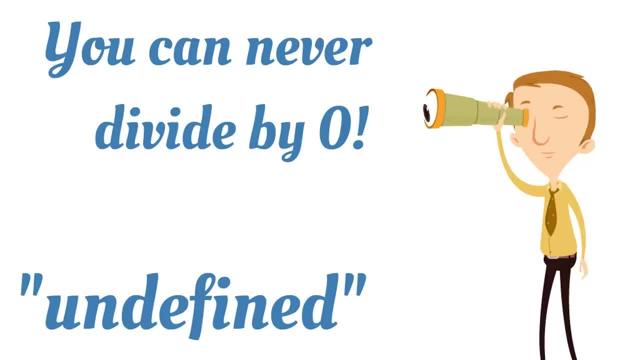 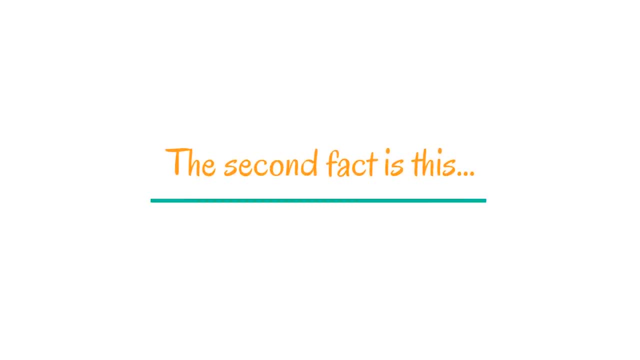 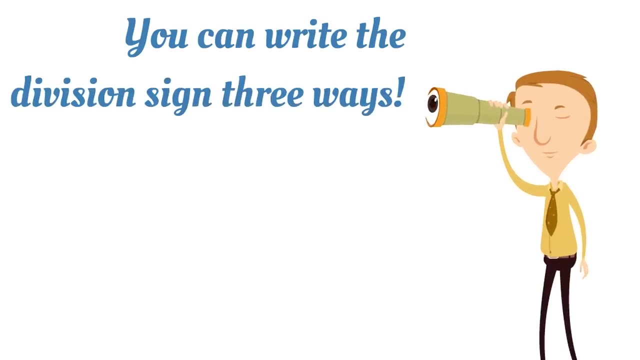 just write undefined. It's impossible. It's impossible, So just write undefined. The second fact is this: You can write the division sign three ways. Uh-huh, Not just with that traditional division sign. You can write it like the division sign. 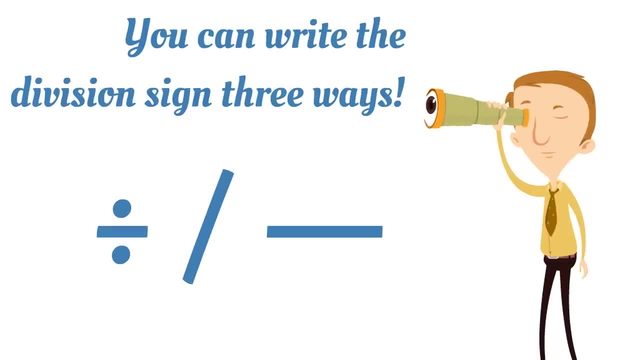 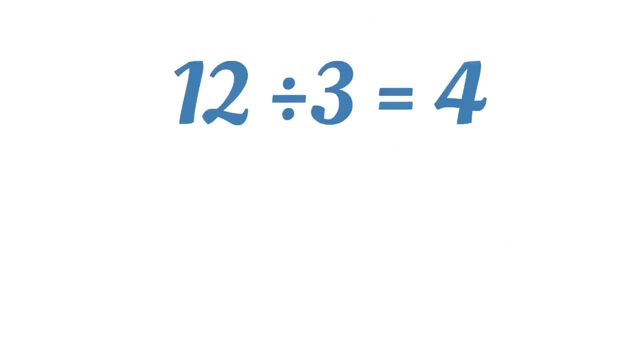 or you can write a division problem with the slash or with a horizontal line, For example. look at this: Twelve divided by three equals four. That's the original division sign, the one that you might see more regularly- Undefined. But here is the same equation written in a different way. 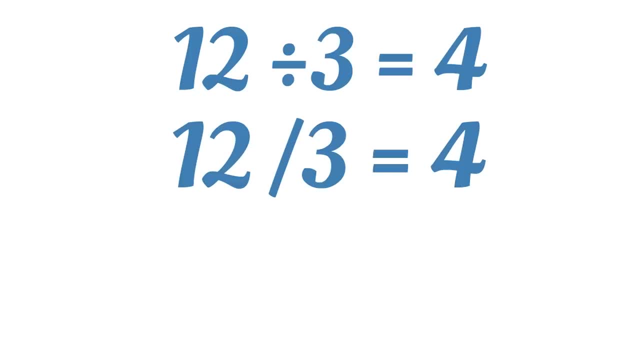 Twelve divided by three equals four. It's still a division sign, but it's a slash. It means the same thing as the original division sign. Remember, the division sign can also be a horizontal line: Twelve divided by three equals four. That looks like a fraction, doesn't it? 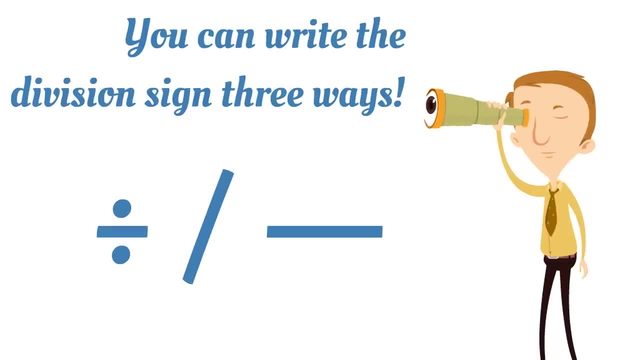 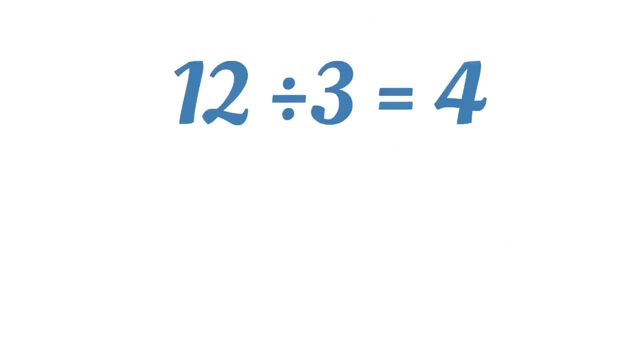 or you can write a division problem with the slash or with a horizontal line, For example. look at this: Twelve divided by three equals four. That's the original division sign, the one that you might see more regularly- Undefined. But here is the same equation written in a different way. 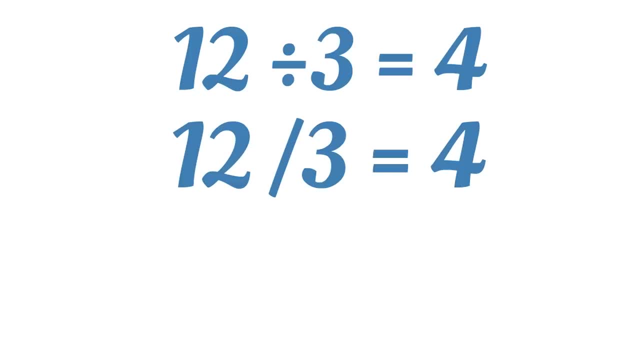 Twelve divided by three equals four. It's still a division sign, but it's a slash. It means the same thing as the original division sign. Remember, the division sign can also be a horizontal line: Twelve divided by three equals four. That looks like a fraction, doesn't it? 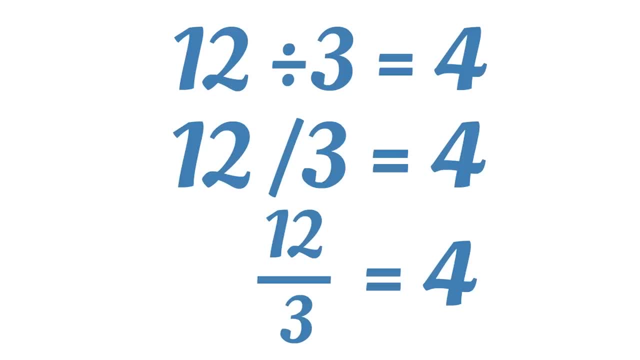 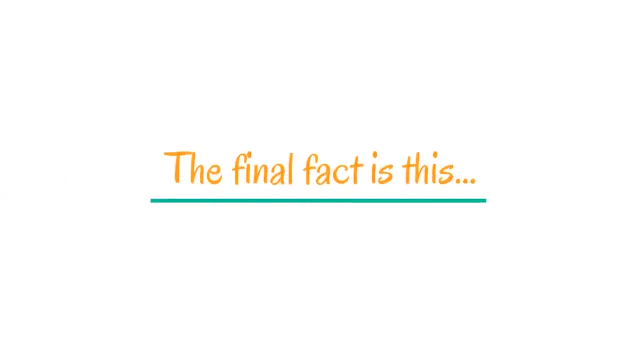 The line in a fraction means divided by. The line in a fraction means divided by. These are the three ways that you can write the division sign. Pretty interesting, All right. the final fact is this: Okay, this is so awesome. You can flip the number of groups and the number in each group. 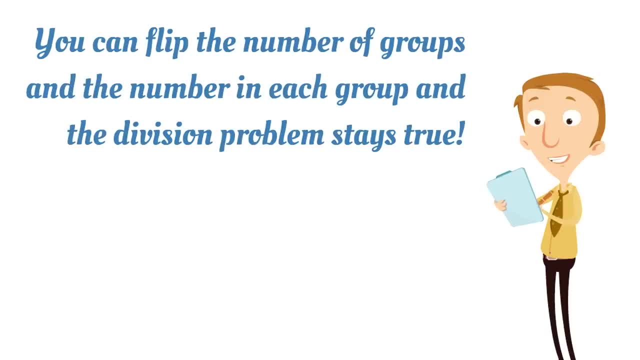 and the division problem stays true. For example, ten divided by two equals five. And you can flip the two and the five and it stays true. That means ten divided by five equals two. Isn't that interesting. Ten divided by two equals five. 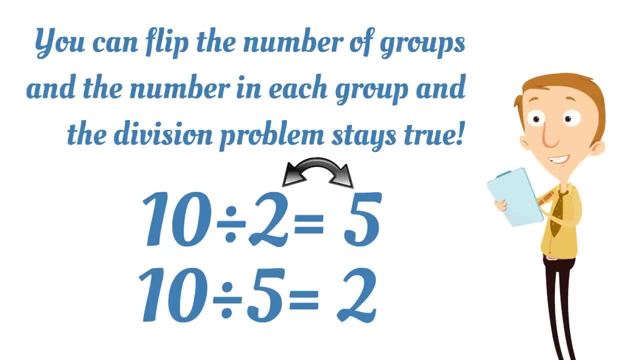 and ten divided by five equals two. You can flip the number of groups and the number in each group and it still stays true. Or look at this: Eighteen divided by six equals three. Remember, we can flip the number of groups and the number in each group. 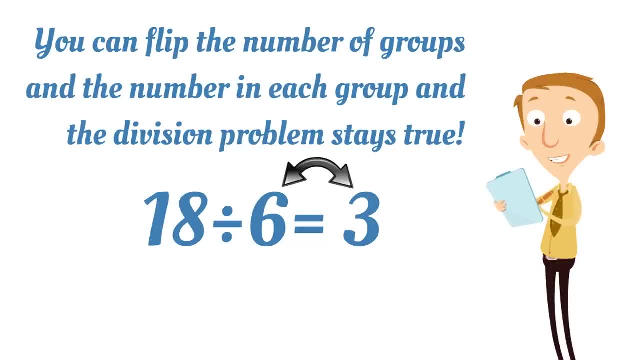 and it still stays true. So we can switch the six and the three, and it stays true. So eighteen divided by three equals six. The six and the three can be flipped. So eighteen divided by six equals three, and eighteen divided by three equals six.